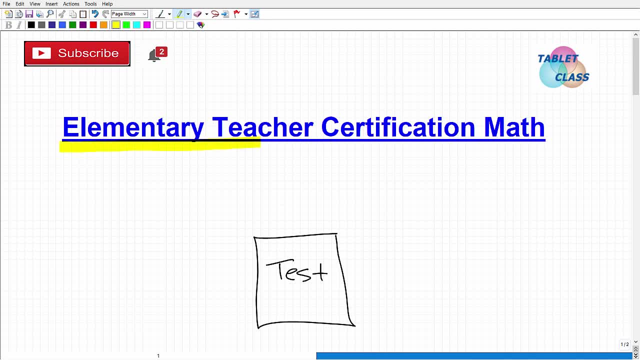 Okay, let's talk about elementary teacher certification, math. Now, this video is just going to be highlighting the type of math that's going to be on most elementary teacher certifications nationally in the United States. Now, this is going to, of course, depend upon what state you're in, okay, what test you're going to be taking, what certification you're going for. So there are some major differences within elementary teacher certification math. 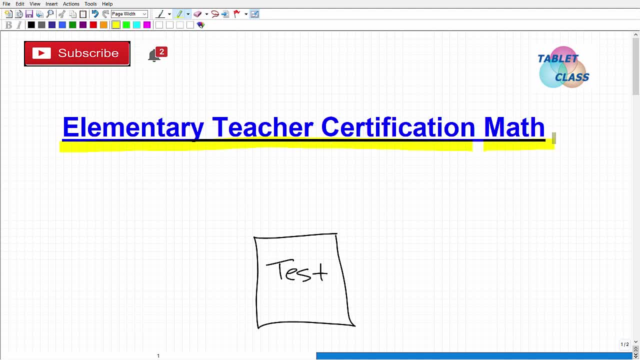 certification exams based upon those factors I just said. But what I'd like to do in this video is just highlight some of the things that are common amongst all these exams and dispel any kind of misconceptions that a lot of people I think have when they are going into elementary teaching, And if they haven't really looked at what's going to be on their certification exams, at least with respect to math, they might be shocked, to say the least. Okay, Now, some of you out 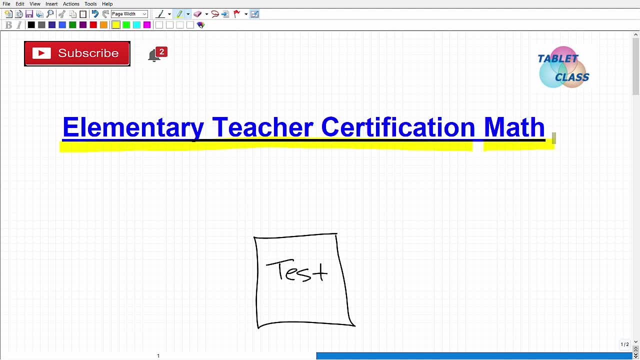 there. maybe that's being a little bit, you know, maybe I'm exaggerating too much, But I do find it that a lot of elementary teachers, you know, when they do look at the math on a lot of exams- a good portion of the certification exams are out there. they are, you know, saying wow, that's a lot more math you know, I need to know than I thought you know to get your elementary teacher certification. So we'll keep this in general terms And hopefully this will help you out. But before we get going, let me introduce. 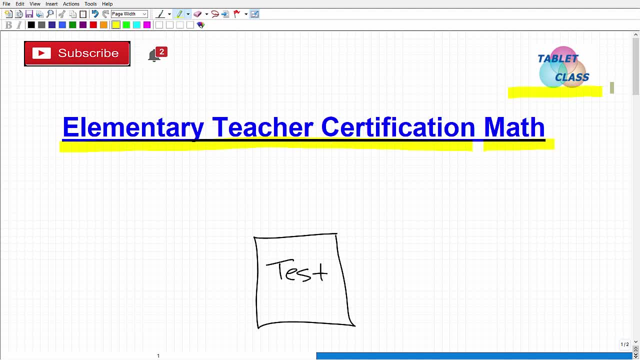 myself. My name is John. I'm the founder of Tablet Class Math. I'm also a middle and high school math teacher. I never taught elementary school. However, I've constructed many, many online math courses. I do a lot of research on what's in these courses And I have several. I have, oh I think it's at least 60- different teacher certification math prep courses. Okay, They've all done very well. I'm going to leave a link to my main math program. 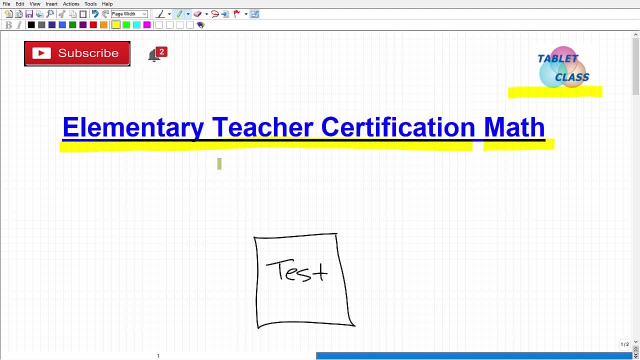 so if you're looking for a specific test that you have to take, obviously you would be right. There is no such thing as an elementary teacher certification general exam. But you know, if you're looking for the practice exam or maybe you're in the state of Arizona, they have their own exam, or Florida, or whatever the case is, I likely have that teacher certification math prep course for you. So again, you could check that out By going to. 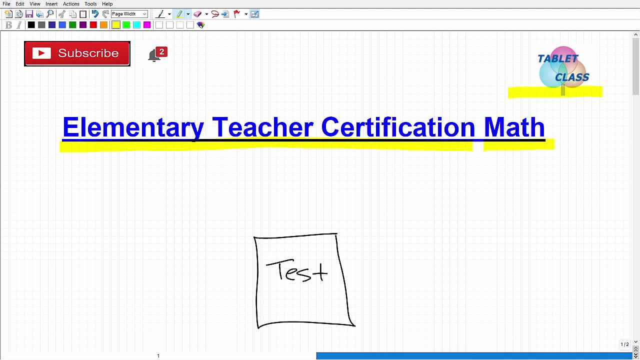 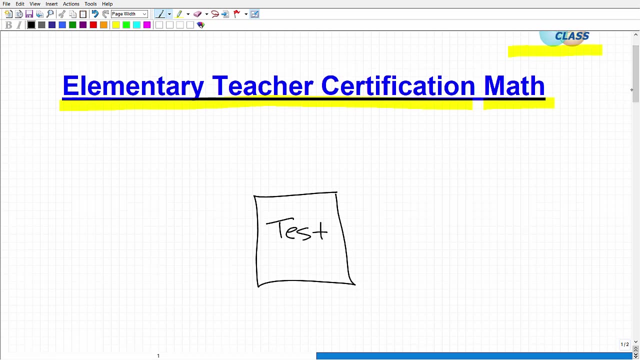 the link in the description of this video and hunting around see if I actually have that test, I probably do. Okay, With that being said, let's get into some main tenets, though, about elementary teacher certification, math. All right, So here is our handy dandy test And some of the things that- and this is again pretty universal- It goes across. it doesn't make a difference what state you're in or what certification. 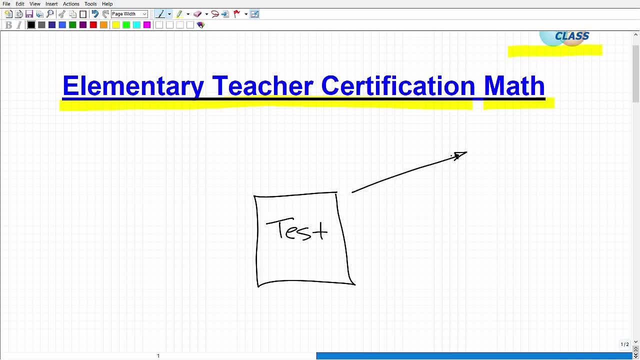 you're going to have, But almost all these tests you're going to need to know way more than just elementary math, Okay. So a lot of teachers and candidates, somebody like: okay, all I need to know is like place value. Okay, like place value is a concept. You know the tens, the hundreds and all that kind of good stuff like that? Yes, you definitely need to know that, And maybe I just need to be really good at fractions and basic geometry. 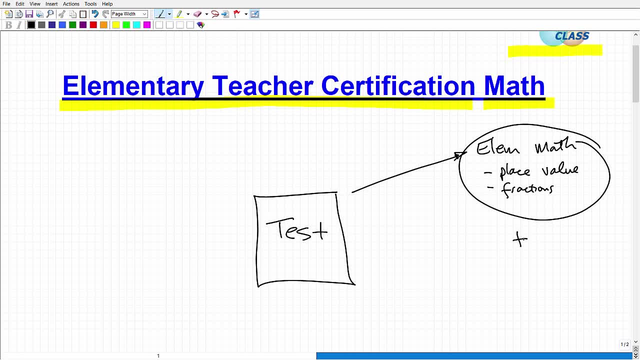 Yes, you need to know all of this. Plus, you're going to need to know what I like to kind of classify as middle and high school level mathematics. Okay, you're going to need to know some algebra and geometry as well, at a pretty good level And, depending upon what teacher, what elementary teacher certification you're going to be going for, you're going to need to know a lot of algebra and geometry. So, right off the bat, if you know, if you leave this video, 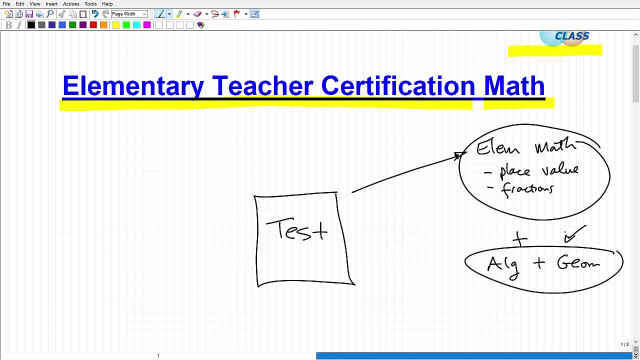 now if the only thing you got out of it is that, hey, you're going to need to know more than just elementary math, you know you're gonna need to know algebra, geometry, then you know. that's one of my main points right off the bat. okay is: don't just because you're going to be an elementary school teacher doesn't mean that for your certification, that's all they're going to test you on. This is very common. For example, as a high school math teacher, right, I had to take the praxis high school of mathematics. 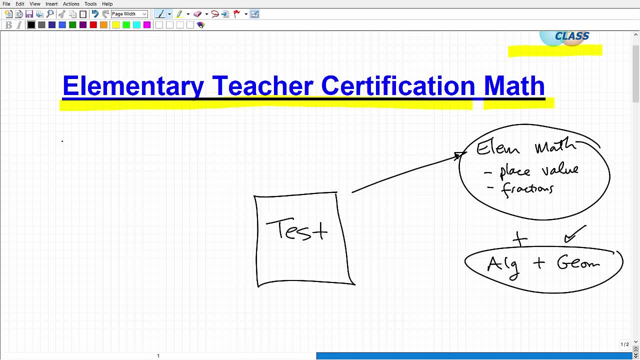 to be able to teach things like algebra two etc. And typically you know this. this can change depending on what state you're in. But let's say you want to be a high school math teacher. you know you'll be teaching algebra two or pre calculus. typically, to have to be a subject matter teacher in high school you can generally have to have a degree you know in that. So most of the teachers that I taught with had a degree you know like a BS in math. 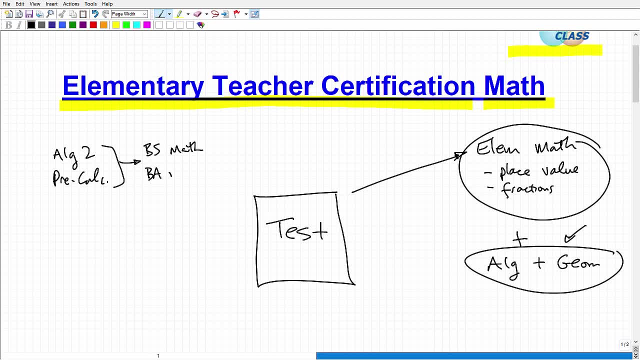 you know, which is a very, very difficult to get- or BA in mathematics- which I have or they'll have- like a math education degree. but then you know they have a degree in that. So if you're like a high school biology teacher, you likely have a biology degree right. So when you take the certification exam to teach you know high school mathematics. you're not just doing basic algebra and geometry, you know high school level stuff. you know they're, they're, you're testing you on calculus, etc. Because 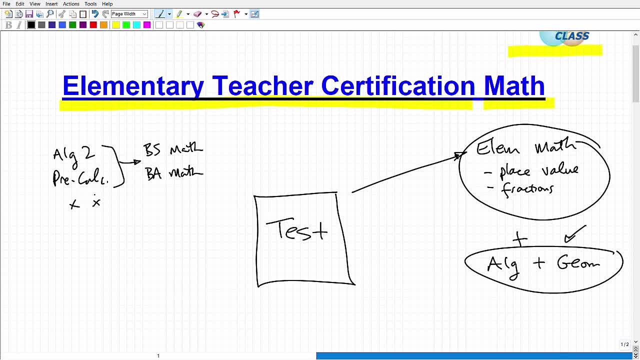 obviously You know you may very well be teaching these subjects at that level. OK, so the certification exams are going to be, you know, testing you on a higher level. Same thing for middle school. middle school mathematics. You know you need to know a lot of more advanced stuff. 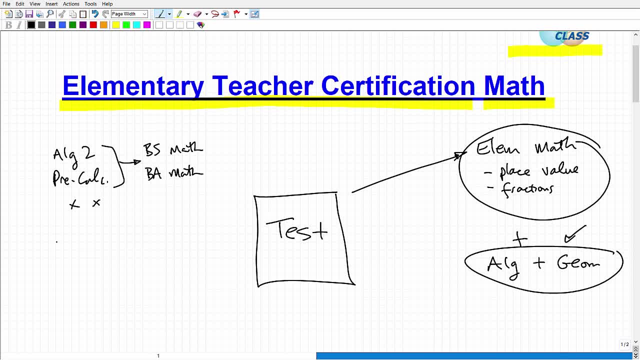 I actually think that's a good way to structure these exams, because you think about it. If you're, you know, an elementary teacher, OK, when you do become an elementary teacher, because I'm sure you will become one- if you're watching this video, you're highly motivated. 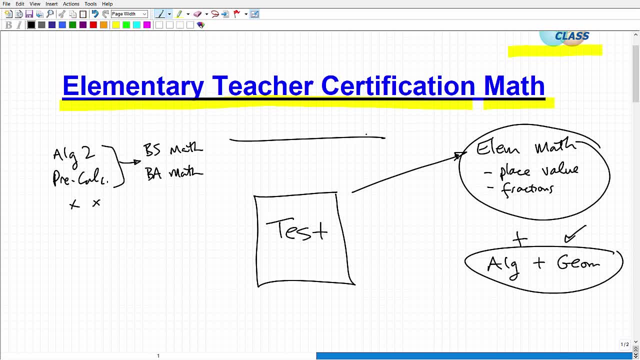 No doubt that you're going to get your certification, But you know education is a continuum. All right. So here's elementary school, Here's middle school, Here's high school. So you are preparing that student to transition into middle school. 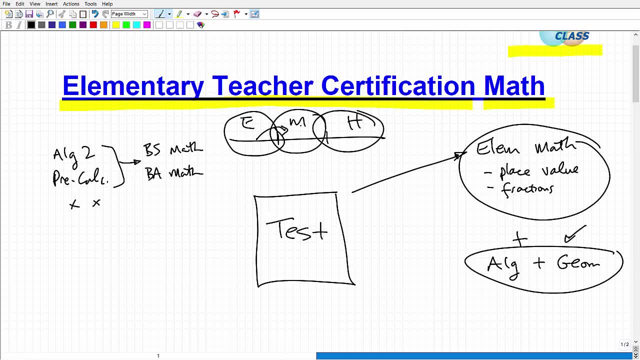 OK, and there's overlap here. So what? When I taught, I taught both middle and high school. You know, I would greatly appreciate the teachers when I taught, like I say, ninth grade algebra, If I had students that were just like really, really good. 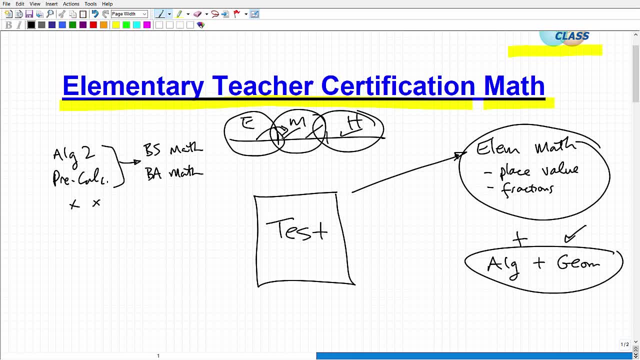 Guess what, I didn't take credit for that. I had to thank all these teachers, especially like in middle school, that prepared them. And then the middle school teachers were like, wow, this, these students were well prepared in elementary school. So they're kind of passing the baton, if you will. 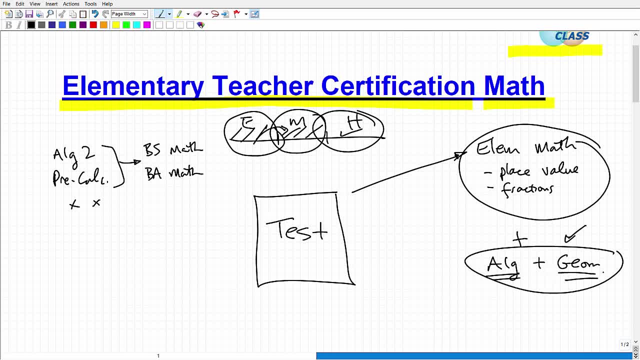 You know, and concepts like algebra concepts and geometry Are being taught at the elementary level. OK, so you need to know a good amount of algebra and geometry for sure. All right, So I would say that's probably the number one thing that you know I really wanted to stress in this video: 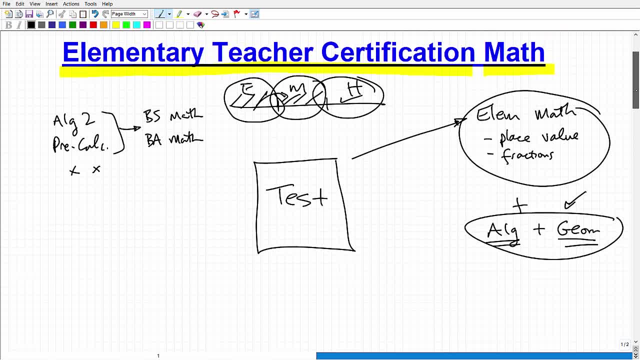 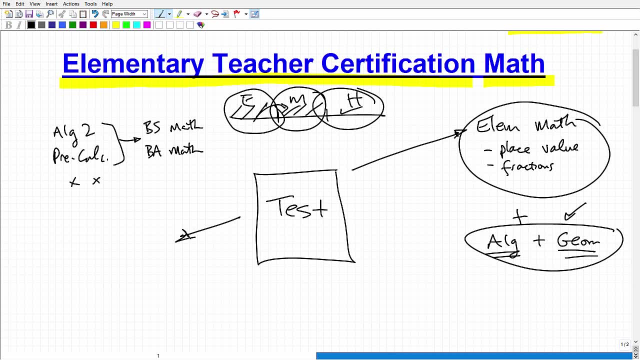 Now I guess the next thing is how you are going to prepare for this exam. So another thing is this kind of goes hand in hand- Is: do you really know what's on your teacher certification exam? So you know what are the objectives. 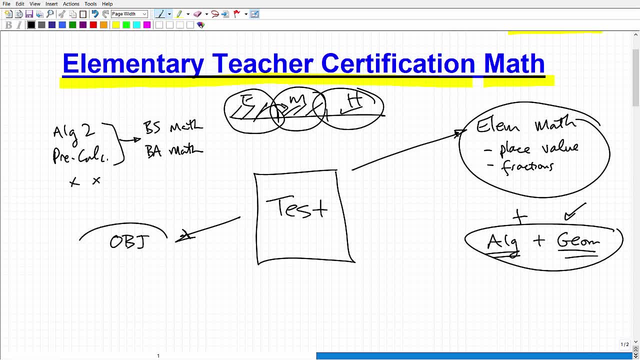 So you can just go to your state Department of Education and look at the specific objectives and you'll see. Hey, you know it depends on what state and what test, but they'll, they'll tell you very specifically. you know, for the most part, you know what math they want you to know. 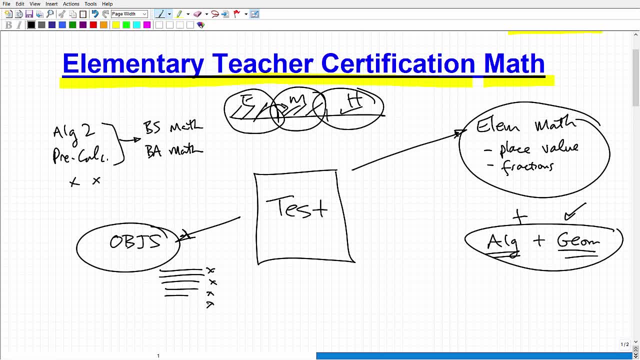 OK, so if there's any question, you can need to kind of do your research, All right. So that's the next thing I want. I want to you know stress, do your research, look at the objectives, look at what you're, you know, required to know. 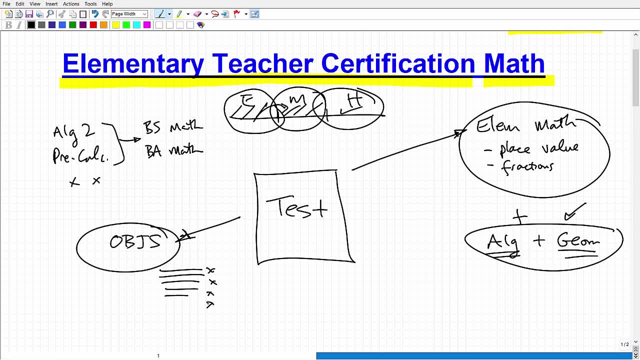 OK, and you do this. you want to have this mindset, you want to do this research so you can put together a good study plan. OK, so a good study plan, you know, is going to be a well-rounded one, All right. 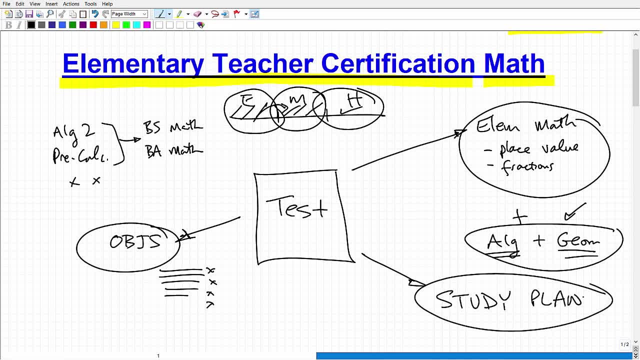 So, study plan, Let's go here. This is your next thing. So I would suggest Using, you know, a hybrid plan. OK, that we don't have to go all in on any one particular thing. you know, kind of diversifies your risk somewhat. 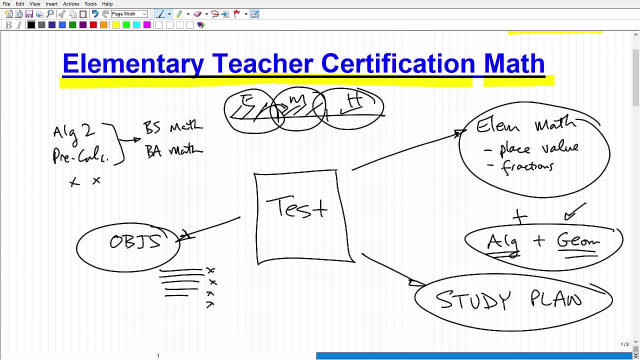 Right. So a hybrid plan would be like: hey, get yourself a good teacher. like a certification for your particular certification, like a study book that has like practice problems and practice exams, Because you know when you're taking a certification exam, it's just you know. you have to know what is the test format. 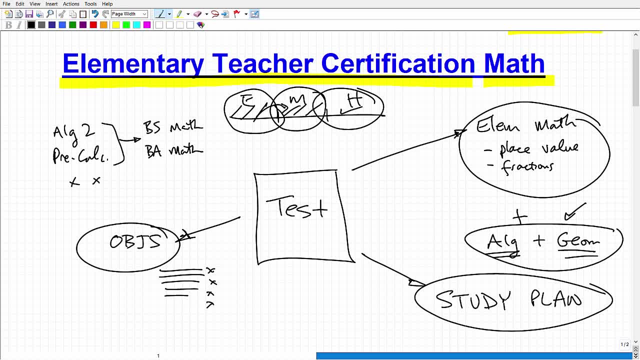 And there's all kinds of different, different approaches. You know you want to get the highest Score, So there's different. We're just talking about test taking strategies and techniques, et cetera. Of course, again, I'm only talking about math. 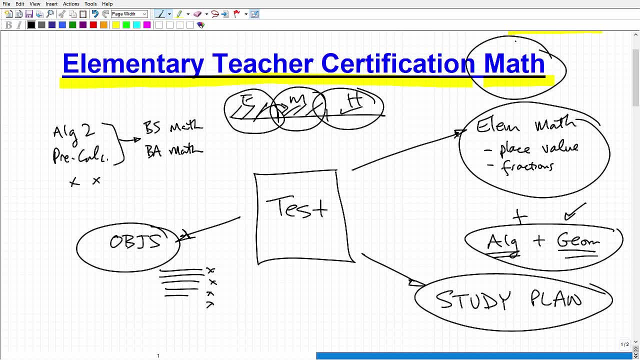 So you want to get yourself a book that's really good on that for sure. Now, when it comes to the math portion of it, you know this is where you have to kind of gauge. you know your current math skills and you know where you're thinking, you're, you're, you're at in math. 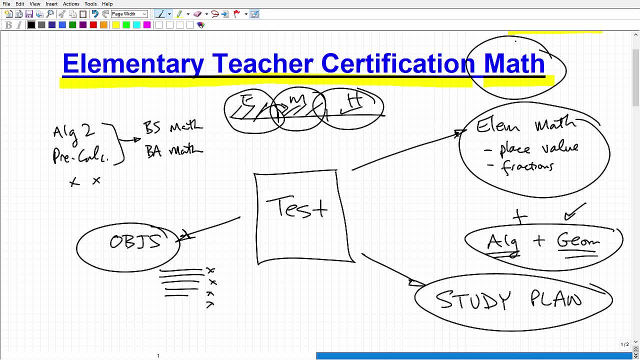 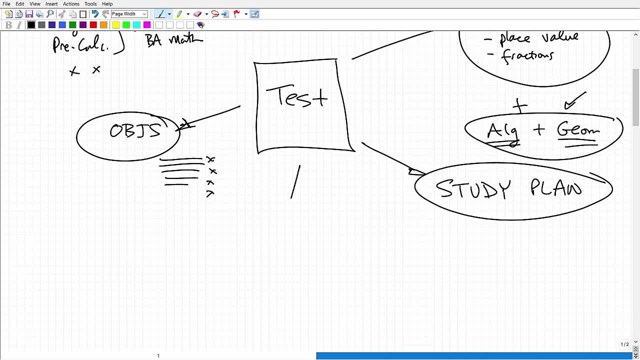 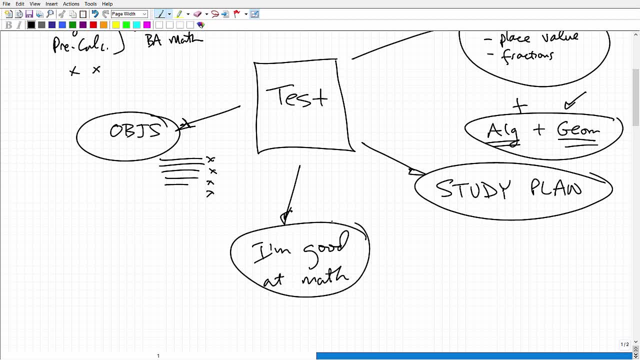 So maybe you are good at math, Maybe you took AP calculus in high school, OK, But then became a elementary school teacher. But guess what? That was four years ago. All right, So let's say, you know, here's four years, or maybe five years. 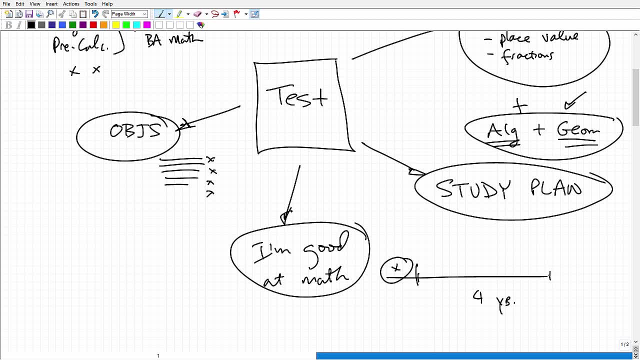 And you took pre calculus and all that good stuff in high school. you know that's a big span of time if you haven't taken math um for a long, long time. in the last math course you took was statistics or something like that. that's not gonna that's not going to. 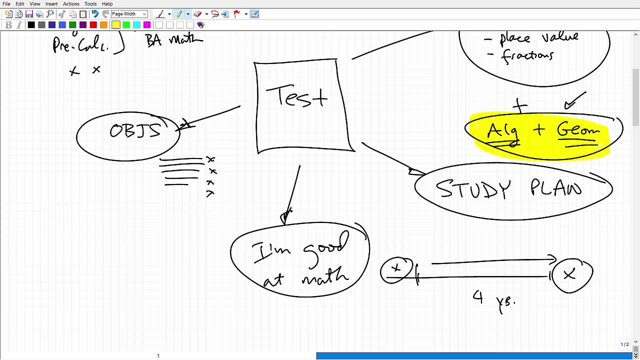 serve you well when you're really going to be asked a lot of high school level, middle school level, algebra and geometry. so just because you're good at math- and i'm, there's no doubt i'm sure you are. if you you were, you know you did good in high school, uh, or in your college courses, that's. 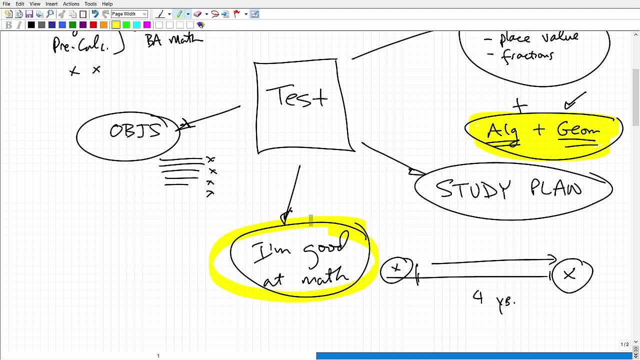 excellent. okay, this is. this should be a lot easier for you, but don't underestimate the importance of you having to review. okay, so you need to review, all right, and you need to review. things are going to be relevant to the objectives, are going to be on this test, so it's not going to be calculus. 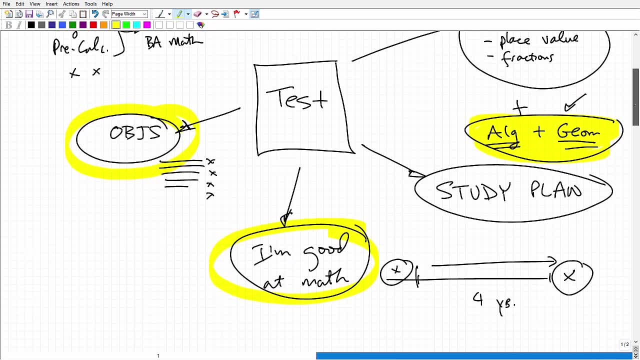 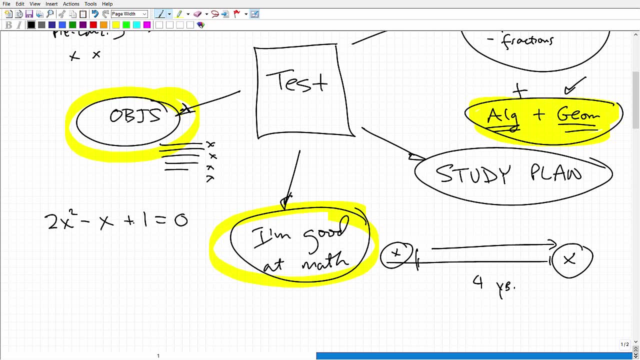 you're not going to be faced with calculus questions on this exam. you know, can you do proms like this? all right, you're like: well, you know it's been a while. well, just because it's been a while, that's not going to. you know, hack it on the test, right, you're going to have to, you know, not be rusty on these math. 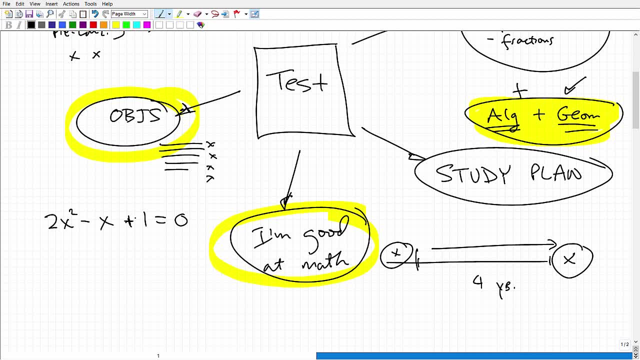 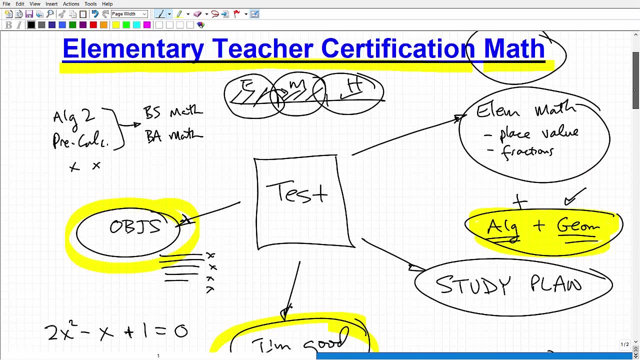 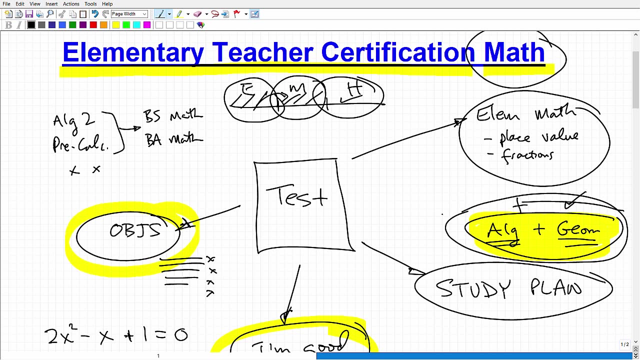 skills. there's a lot of math skills that you're going to have to kind of refresh, and that's the last thing i want to. um, i remind you is that for the elementary level certification, all of you have passed the math that you're going to need to um know for this test. okay, it's just uh, back in. 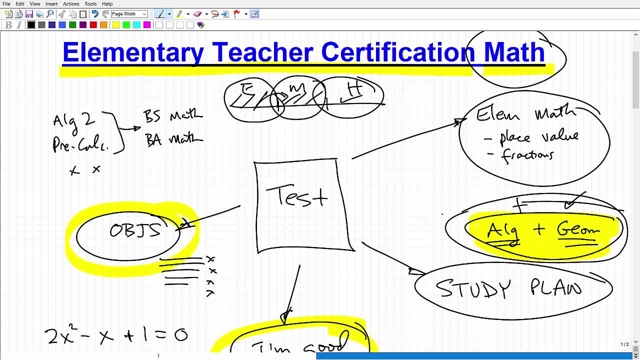 you know recesses of your mind and you wouldn't be where you're at. if you're getting ready to take your teacher certification exam, you wouldn't be likely a college graduate or getting ready to to graduate. you've already been very successful academically. you're highly motivated, committed. you know all. 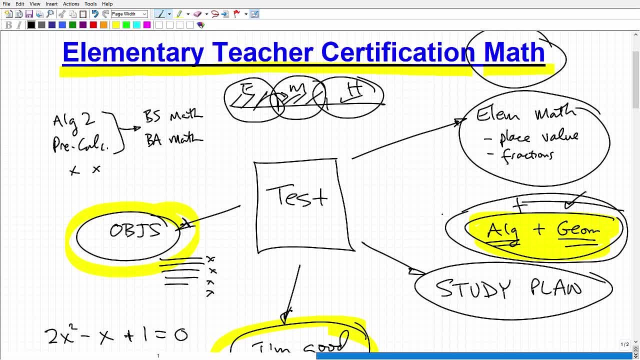 those things you have. okay, uh, you know how to study, etc. but what you do need to do is to kind of organize your battle plan here so you can take this test the first time. so if you're new to i can tell you right now teachers fail certification exams quite frequently. right, there are some. 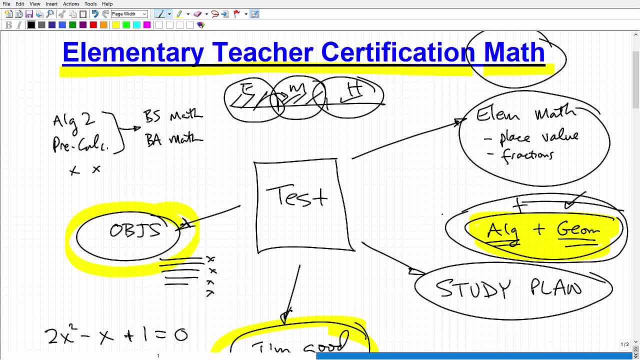 teachers out there that have been taking tests for years trying to pass them and that sounds kind of like crazy, but i'm telling you right now: um, lots and lots and lots of teachers in all states with various different certifications that have been struggling to get their certification and 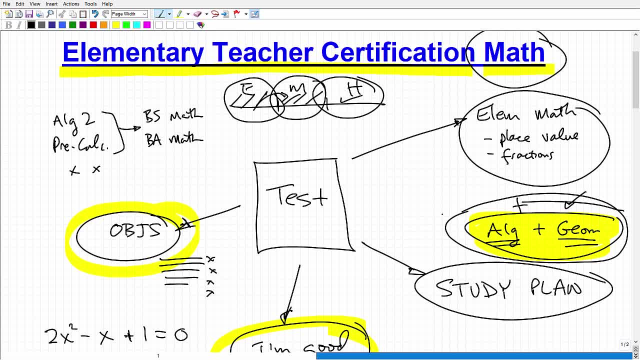 pass these tests. so don't underestimate. you know the importance of, of having an organized, you know, smart, intelligent plan. okay, now, of course, getting your elementary teacher certification. there's other topics, not just math, in there, but of course this is just related to math, as math is one of those topics that tend to be, you know, give a lot of people trouble all. 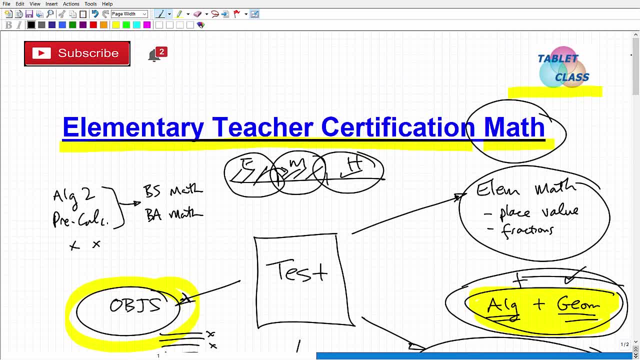 right, so let me go ahead and wrap up this video again. there are several elementary teacher certification exams out there. uh, within you know, some states might have two, three, four different types of exams, and the math can vary quite a bit, by the well, by the way, too, uh, depending.